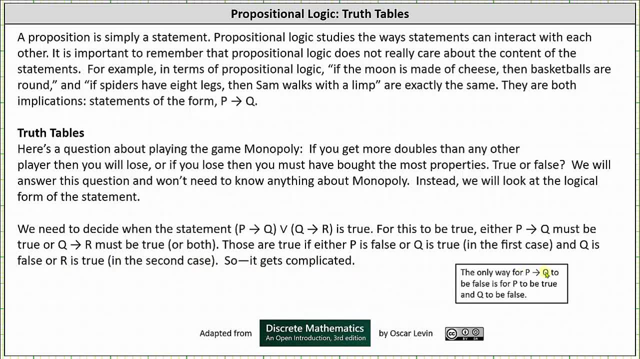 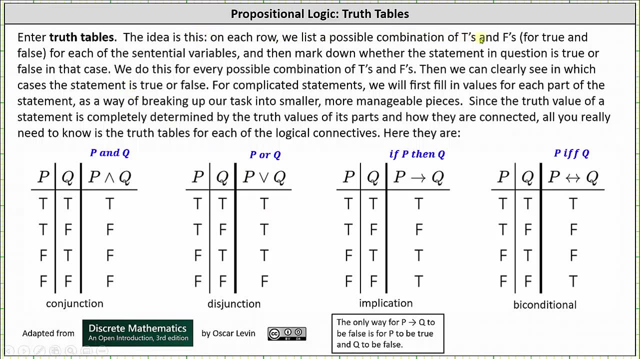 Remember, the only way an implication in the form of if p, then q is false is for p to be true and q to be false. This is where truth tables enter. The idea is this: On each row, we list a possible combination of t's and f's for true and false for each of the 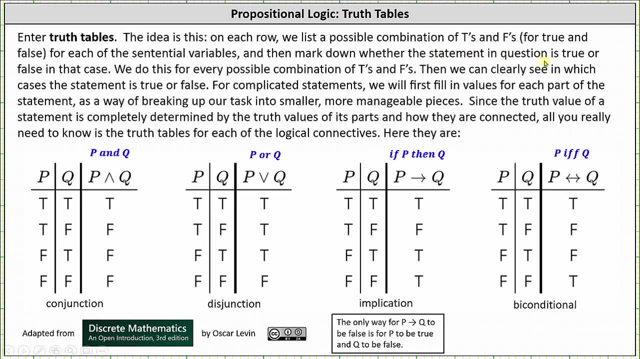 sentential variables and then mark down whether the statement in question is true or false. in that case We do this for every possible combination of t's and f's. Then we can clearly see in which cases the statement is true or false. For complicated statements, we will first 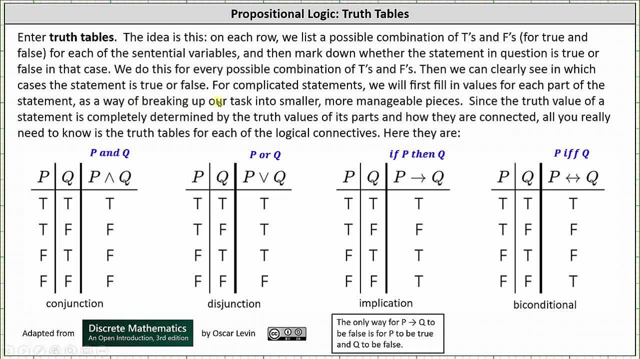 fill in the values for each part of the statement as a way of breaking up our task into smaller, more manageable pieces. Since the truth value of a statement is completely determined by the truth values of its parts and how they are connected, all we really need to 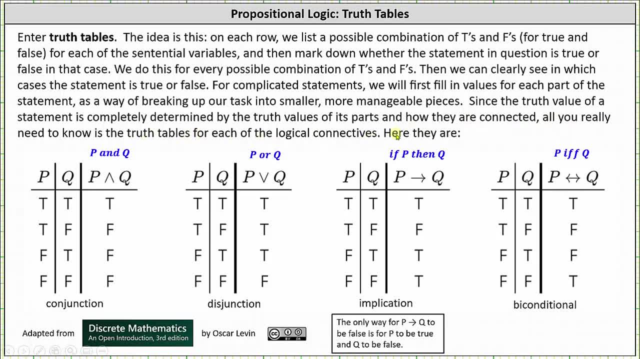 know is the truth tables for each of the logical connectives. And here they are. To begin notice, the first two columns of all the truth tables are the same. They list all the possible combinations of t's and f's. for p and q We have true, true, true, false, false, true and false, false. First, 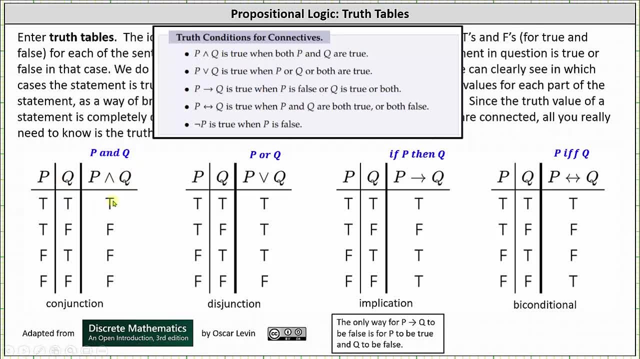 p and q is true when p is true and q is true. otherwise, p and q is false. Next we have the truth table for p or q. p or q is false only when p is false and q is false. otherwise, p or q is true. 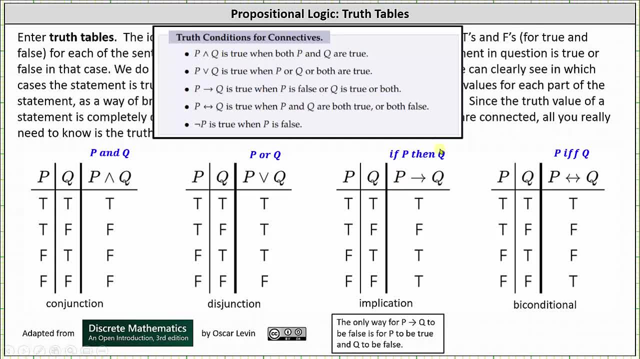 Next we have the truth table, for if p, then q, If p, then q is false. only when p is true and q is false. we see here in the second row. otherwise, if p, then q is true And on the far right we have the truth. 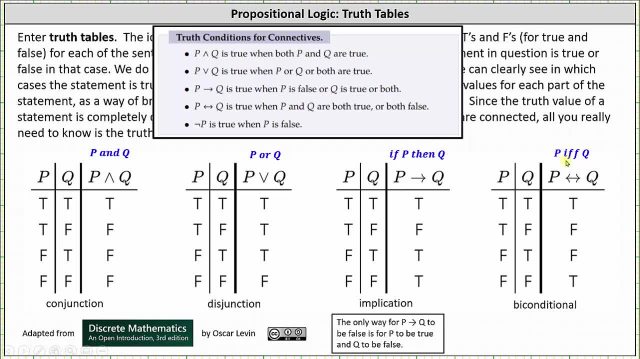 table for: p if and only if q, p if and only if q is true. when p is q and q is true, or when p is false and q is false. otherwise. p if and only if q is false. It's extremely important that we have a 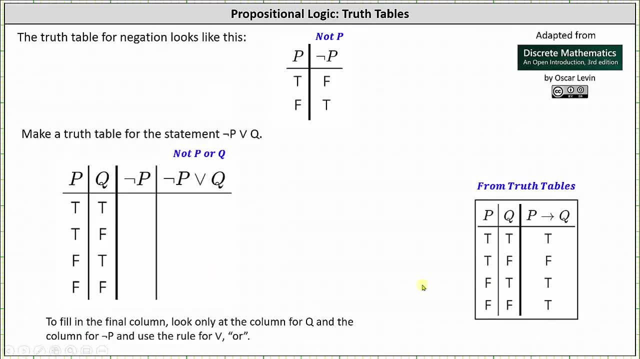 good understanding of these four truth tables. In addition, here's the truth table for the negation of p or not p, Not p, or the negation of p is false when p is true, and the negation of p or not p is true when p is false. And now let's make a truth table for the statement, the negation of p or q. 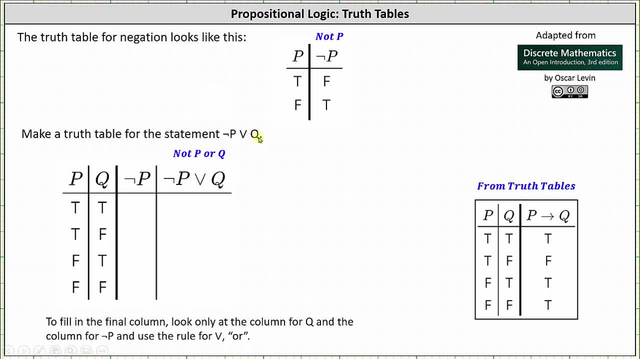 or we can say not p or q. Again, the first two columns list all the possible combinations of t's and f's for p and q. And now let's complete the column for not p. Not p is false when p is true and not p is true when f is true. 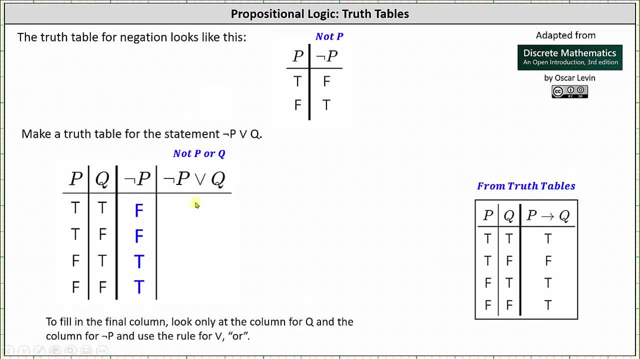 p is false To fill in the final column. we look only at the column for q and the column for not p and we use the rule for disjunction or or. The only way not p or q can be false is if not, p is false and q is false. Notice, in the second row, not p is. 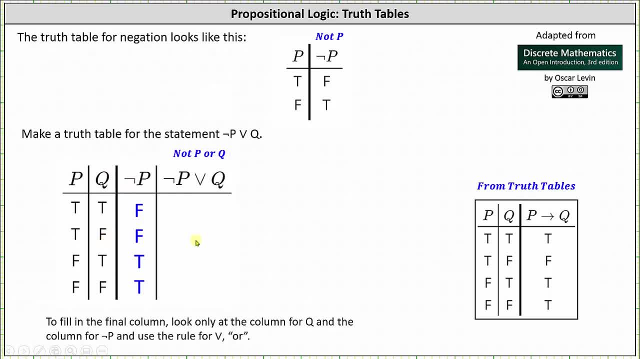 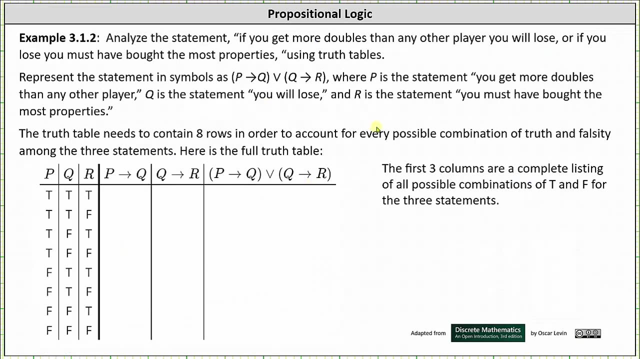 false and q is false. and therefore in the second row, not p or q is false. everywhere else, not p or q is true. Here's the complete truth table for not p or q. And now let's go back to the monopoly question. Let's analyze the statement. if you get more doubles, 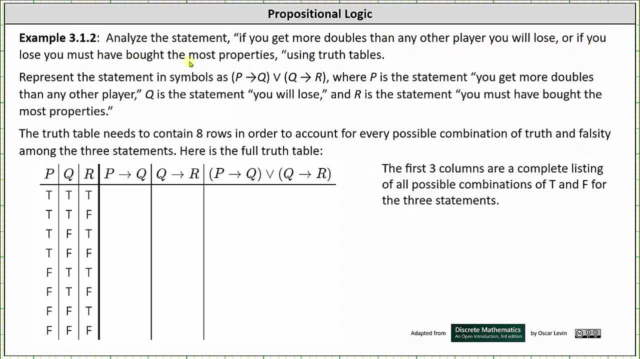 than any other player, you will lose, or if you lose, you must have bought the most properties. using truth tables Represent the statement in symbols, as if p then q or if q then r. where p is the statement, you get more doubles than any other player. 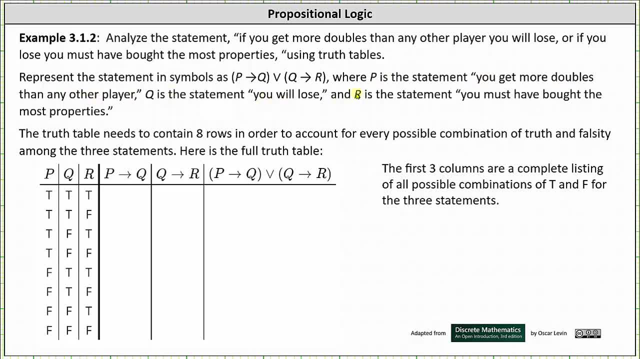 q is a statement you will lose and r is a statement you must have bought the most properties. The truth table needs to contain eight rows in order to account for every possible combination of truth or falsity among the three statements. Notice the possible combinations of truth or. 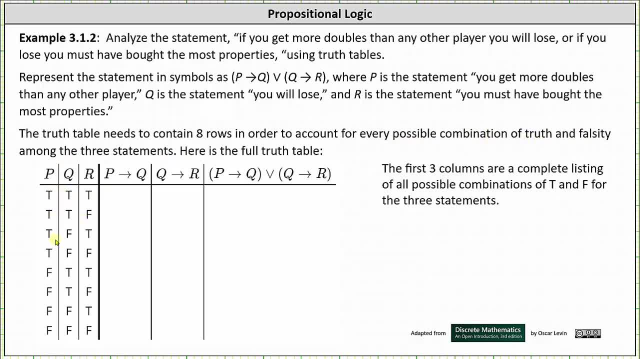 falsity are true, true, true, true, true, false, true, false, true, true, false, false, false, true, true, false, true, false, false, false, true and false, false, false. If p, then q is false only when p is true and q is false. 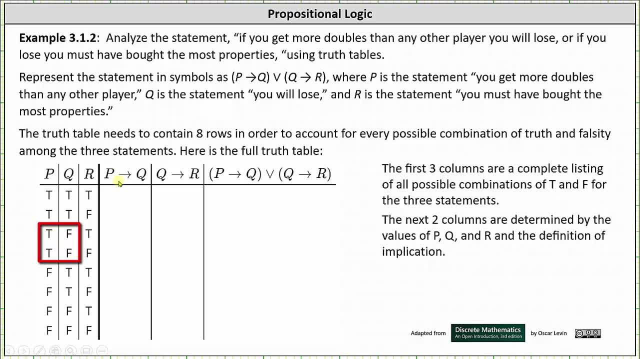 notice that occurs in row three and row four. everywhere else. if p, then q is true. If q, then r is false. only when q is true and r is false. notice q is true and r is false in row two and row six. everywhere else, if q, then r is true.